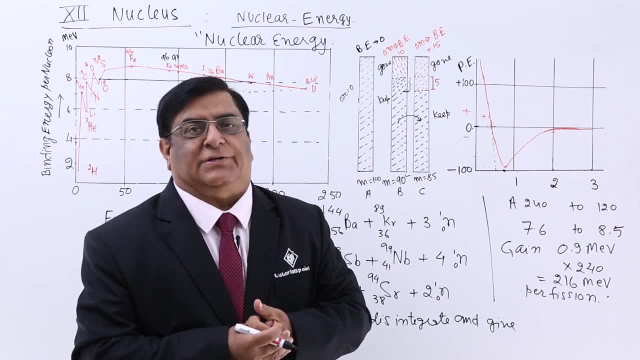 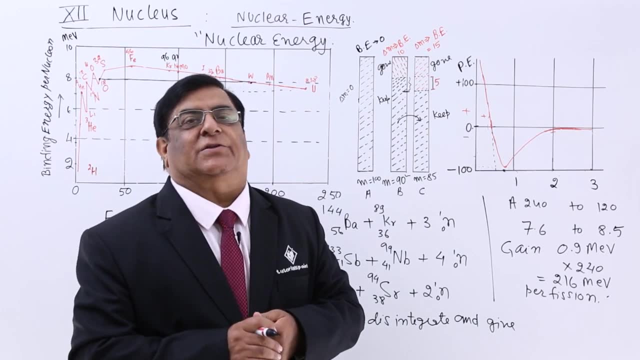 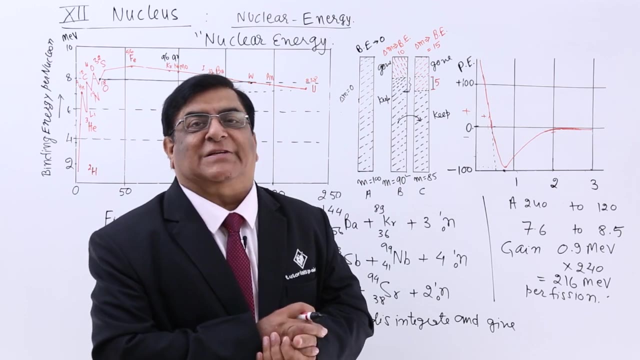 That energy, which is nuclear energy, is very high in quantity. It is almost 10 to the power, 7 times. Then the thermal energy or the chemical energy we receive from the other sources, like coal. One kg of coal gives 10 to the power, 7 joules. but one kg of uranium gives us 10 to the power. 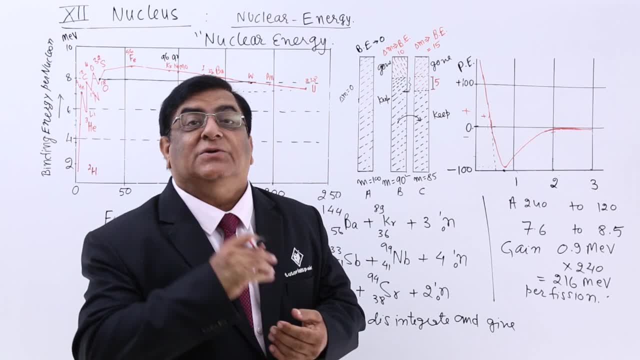 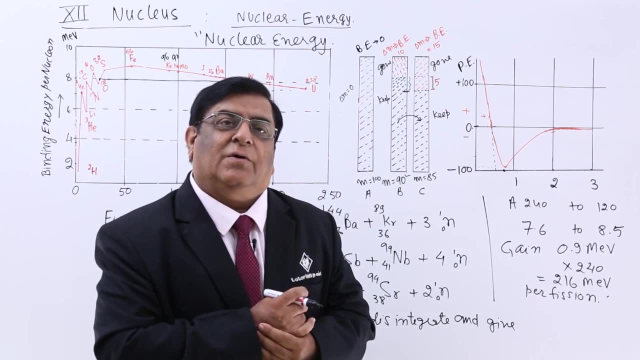 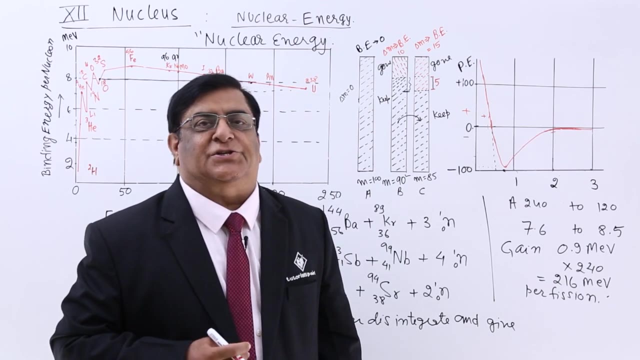 14 joules, 10 to the power, 7 times more than the coal. So nuclear energy is very beneficial in that sense. Now what we are studying is what happens inside the nucleus. So what we do initially is: first we will see the process of fission. In fission we 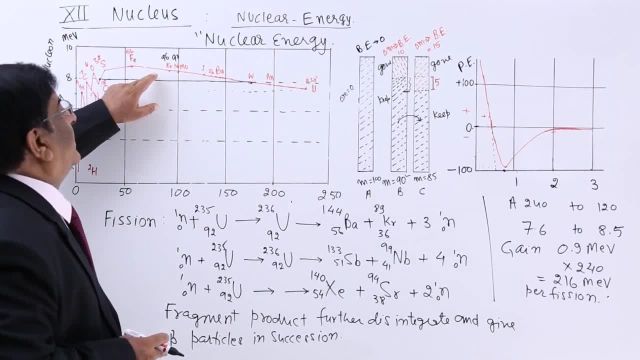 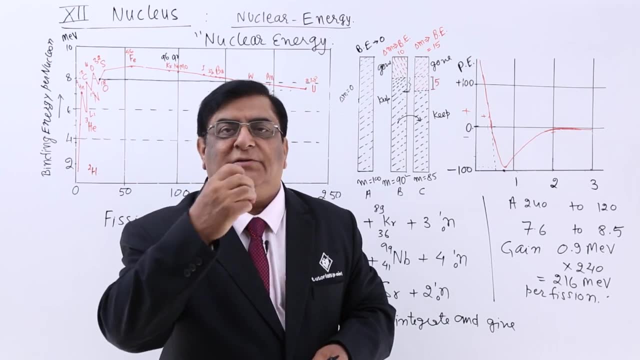 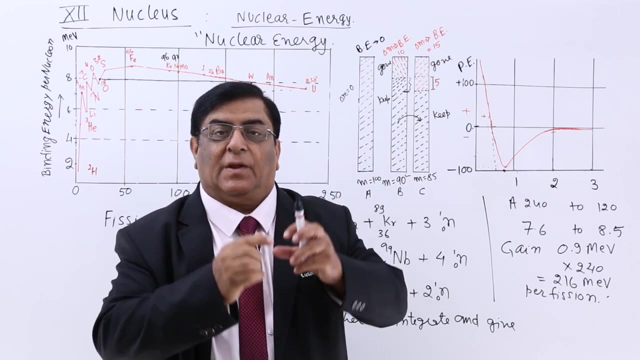 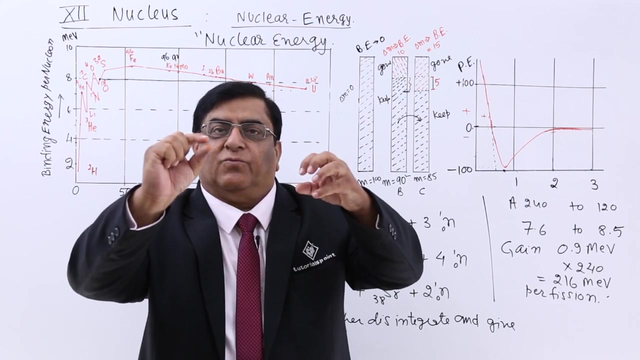 break a large nucleus into two smaller nucleus. Now what is the process of breaking it? The process is we get the nuclear uranium- large one- and we fire one neutron in it. neutron, What will it do? This is the large one nucleus of uranium and one neutron enters it. When one neutron enters, 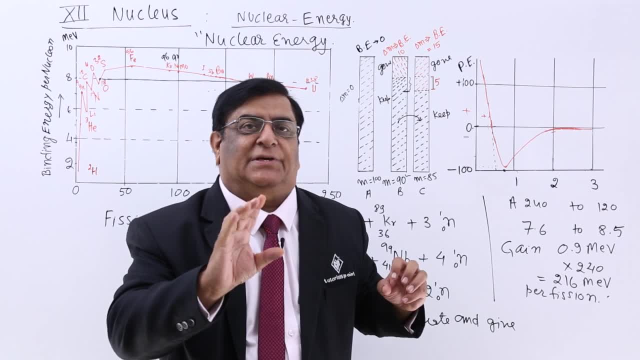 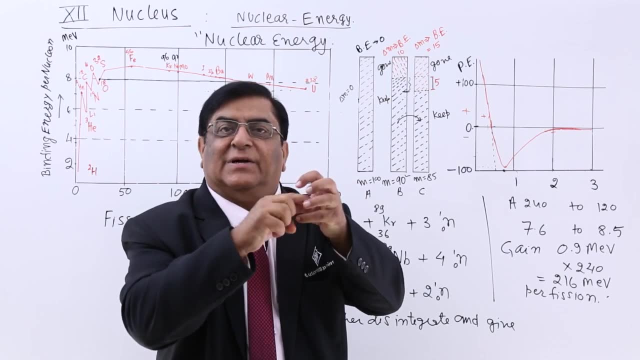 it. it has got only that much energy. We choose such a neutron that it has only that much energy that it can enter in it, but it cannot exit. It will not exit only that small energy. So we call it thermal neutron. 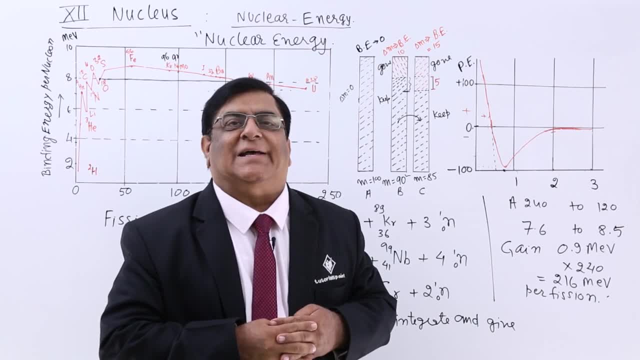 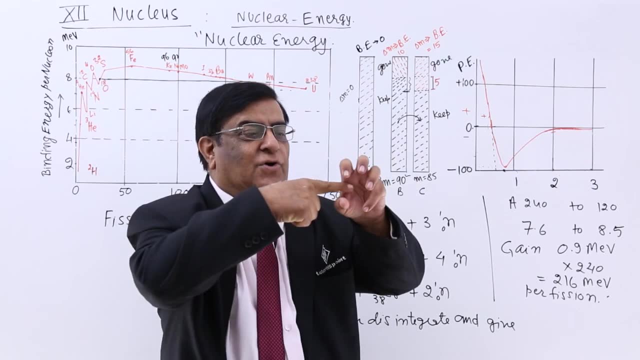 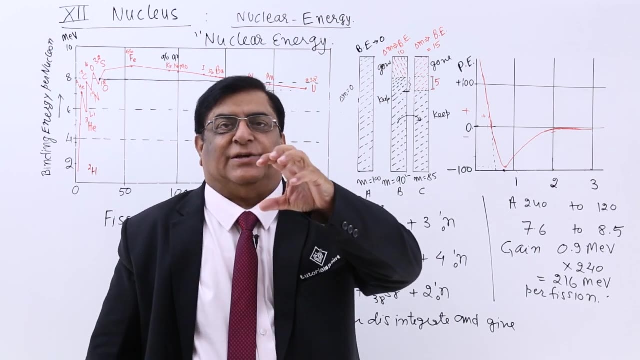 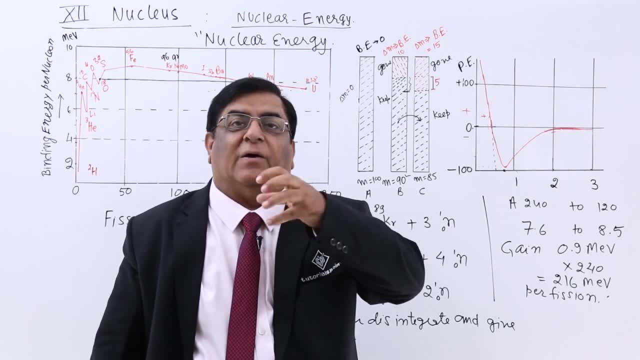 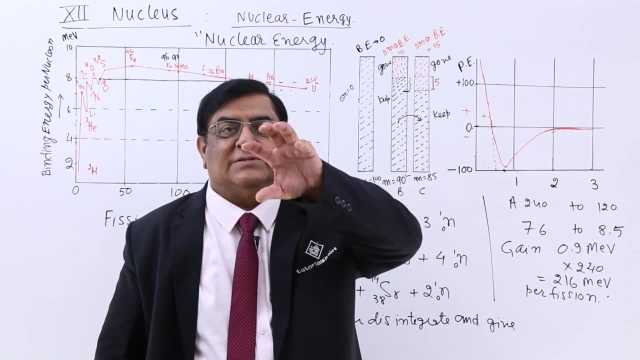 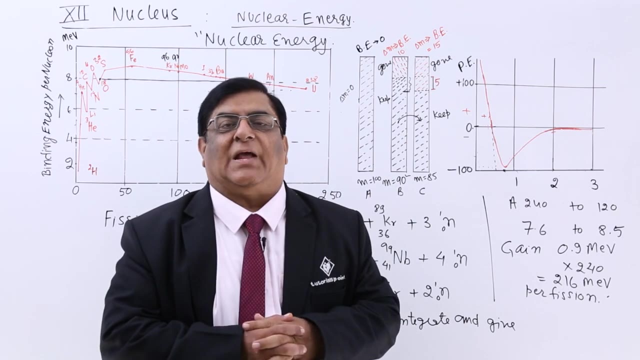 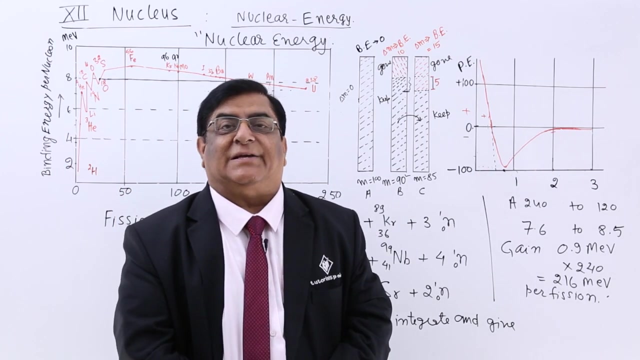 Now, when the size increases, we have studied that nuclear forces become weak. When the nuclear forces become weak, then what happens? If the nuclear forces, the binding forces, become weak, this nucleus breaks and it is trying to balance and finally it breaks up and it breaks up. 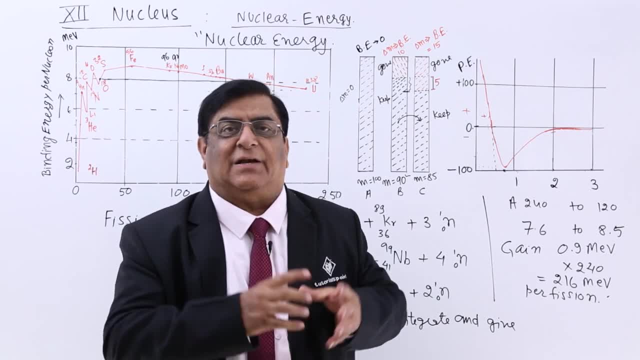 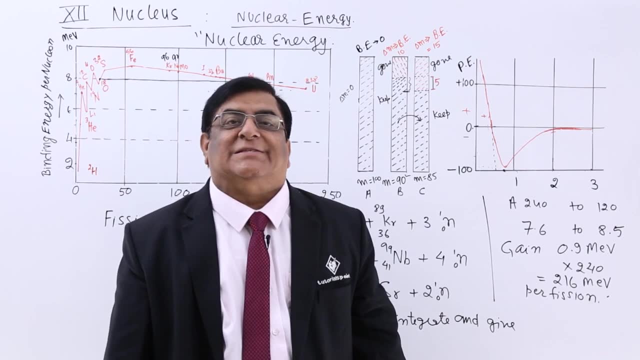 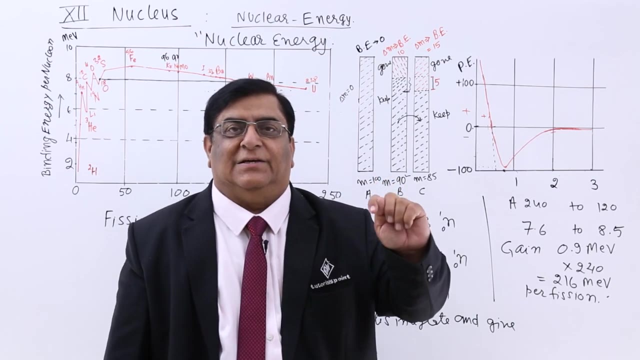 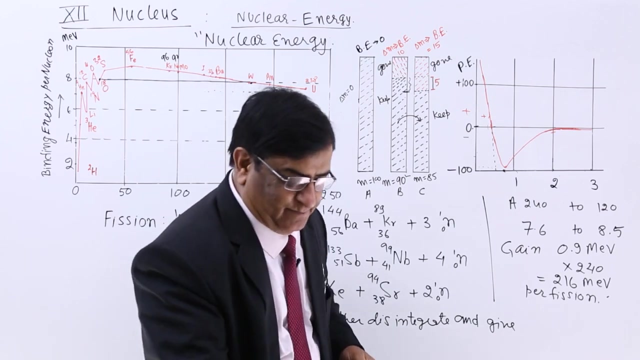 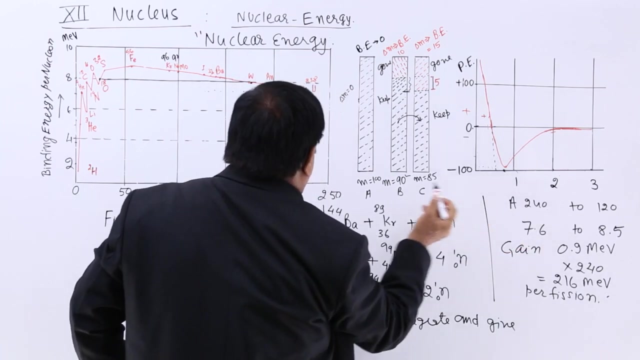 into many fragments. basically, it breaks up into two large fragments. This two large fragments, the size is decided by itself. we cannot order it or we cannot design it. that what should be the size of these two fragments? Now, when this breakage is there, what happens? see, this has got energy at the atomic number. 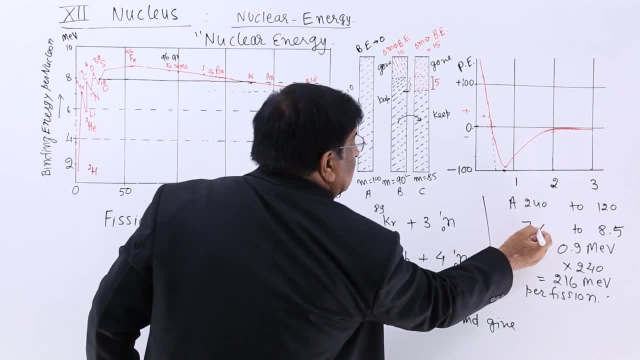 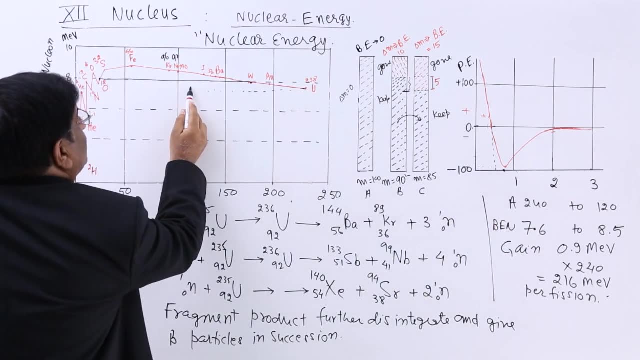 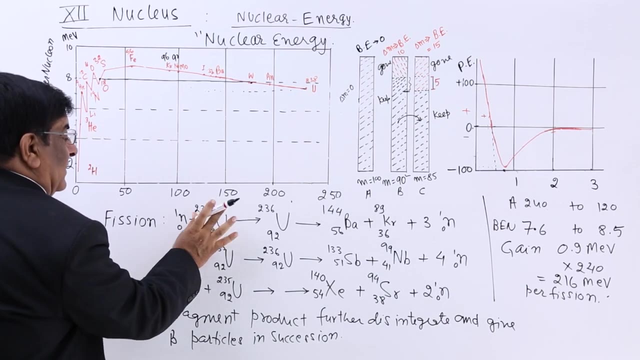 240 approximately. the energy is 7.6 binding energy. it breaks into two parts. what is the reaction? Here is the reaction. Here is the reaction. This uranium we take, the most suitable uranium for this action is uranium-235.. 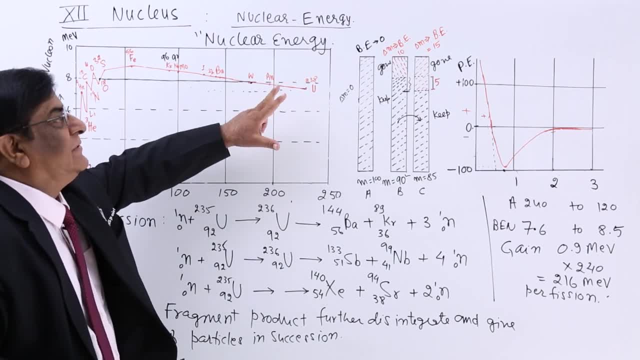 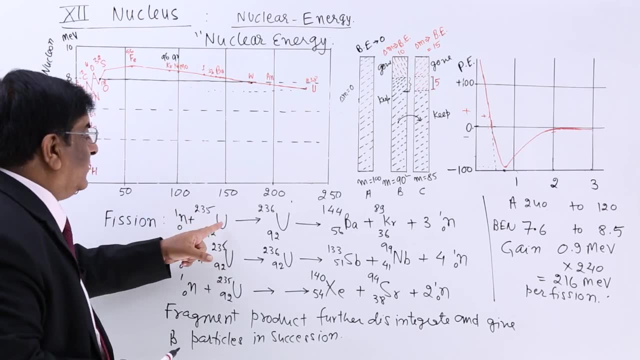 In 238, we find it difficult to do the experiment and we found that 235 uranium is very much suitable for it. So we take 235 and bombard it with one neutron. then this one neutron enters and its mass increase from 235 to 236. 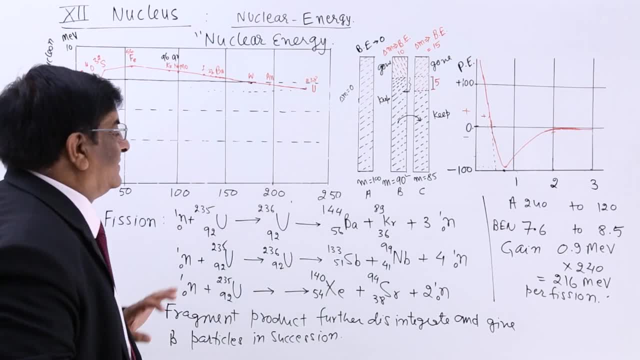 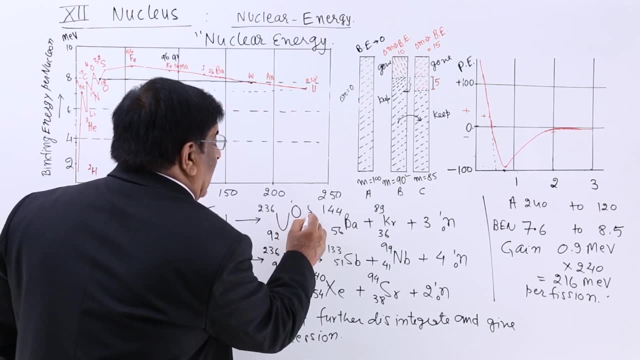 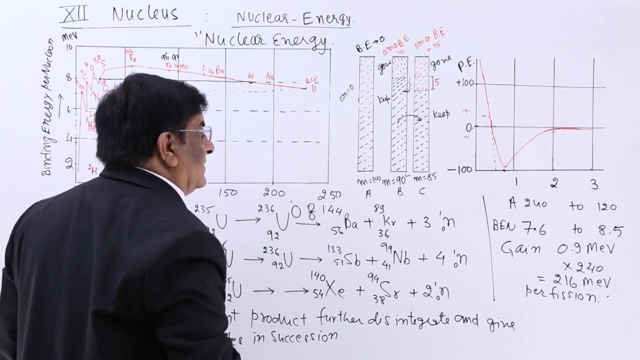 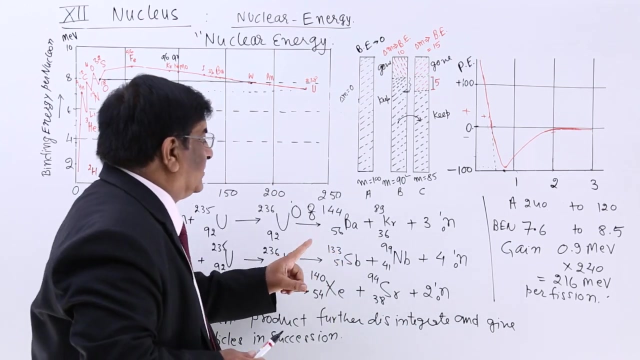 It has become an unstable nucleus. This unstable nucleus, finally this become very large and it breaks into two. a neck develops and it breaks into two parts. Some nucleus break into two parts, which are barium and krypton. Some nucleus break into two parts. 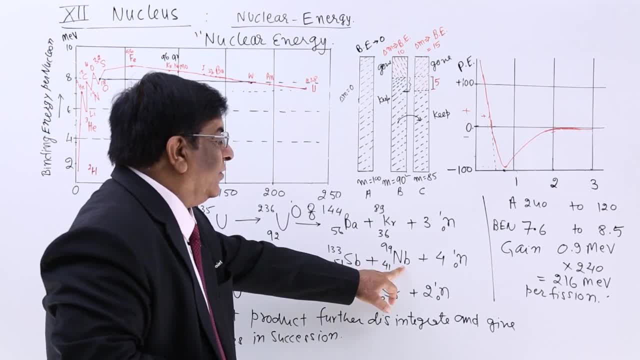 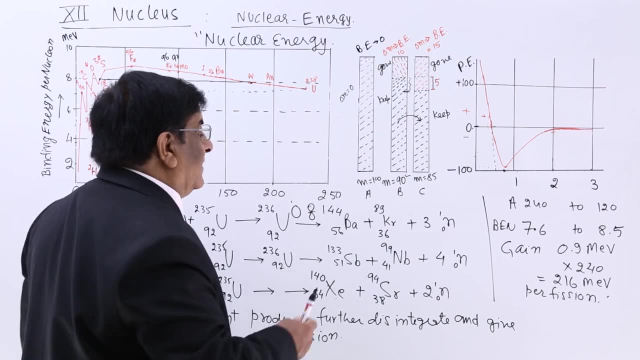 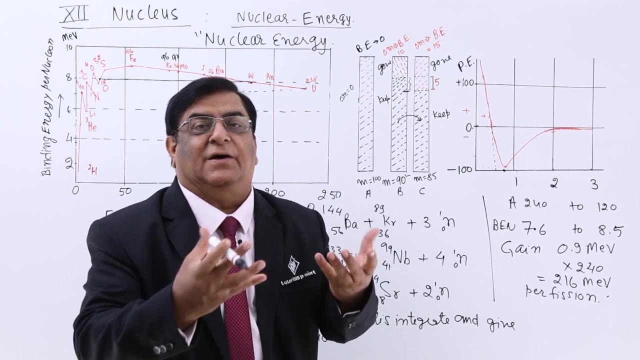 Some nucleus break into two parts. Some nucleus break into two parts: Sb and niobium, Nb. some break into two parts: xenon and Sr. We find so much: barium, krypton, Sp, Nb, Xc, Sr, all parts we find after this break up. 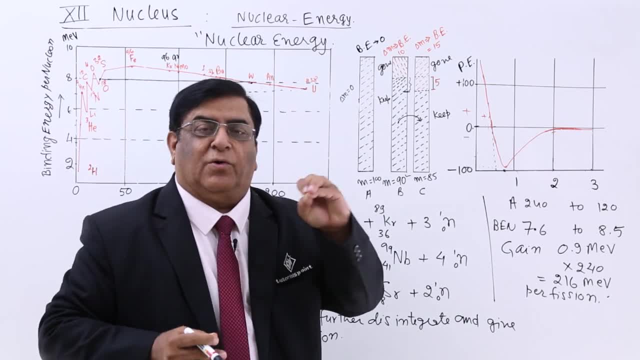 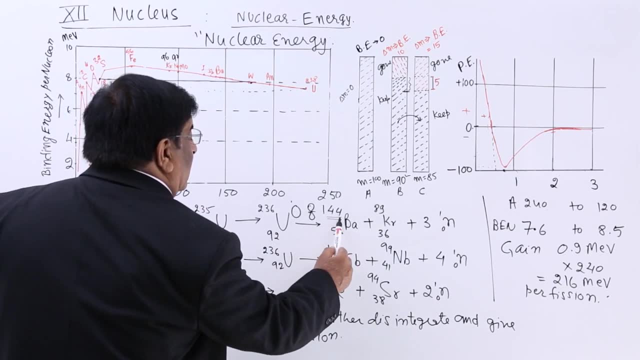 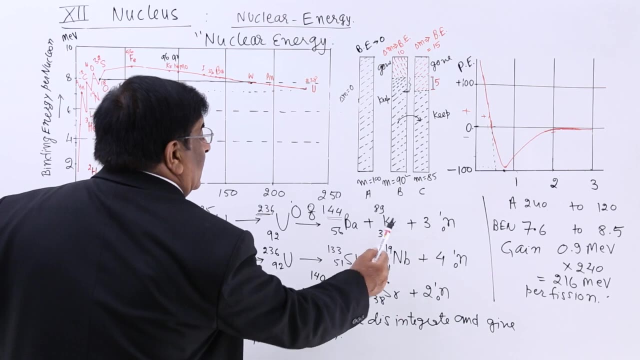 And we make equation by our own combination and calculations. How do we calculate That if one part is barium-144, the total breakage was 236.. Then we can assume the other one must be krypton, because 56 plus 36 is 92.. 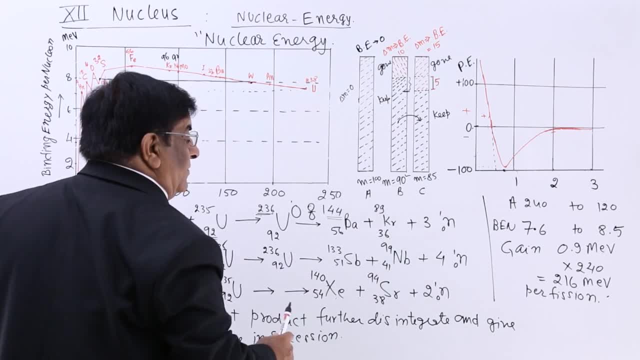 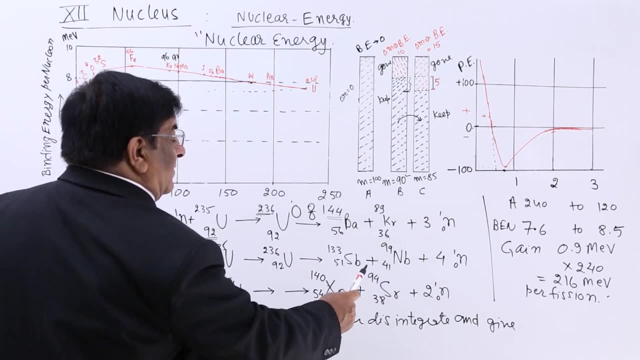 So what is the counterpart of barium-krypton? What should be the counterpart of Sb? If Sb is 51, the counterpart should be niobium, because these two will make 92. Its counterpart cannot be this. Its counterpart cannot be this. 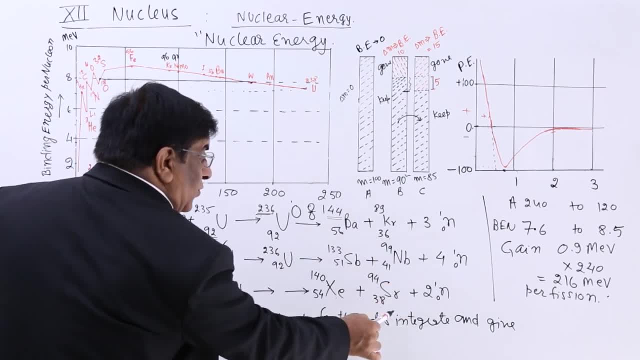 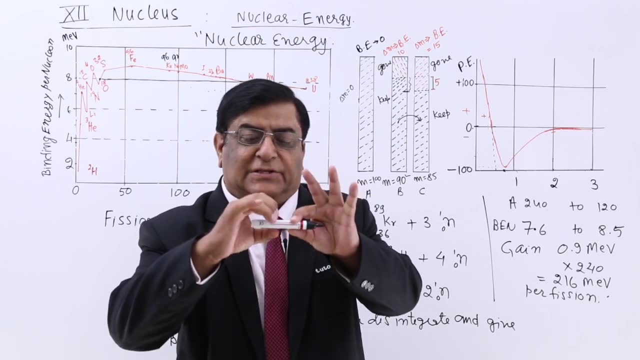 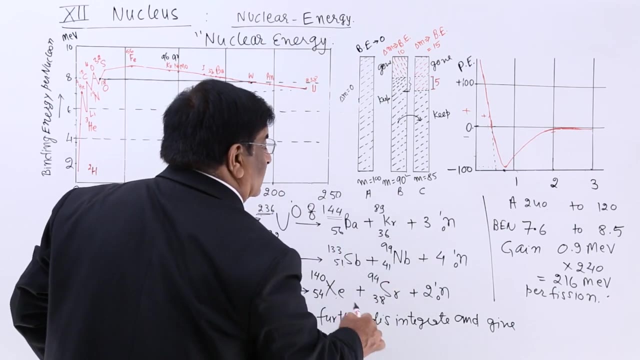 So we set our self, That is, we are receiving so many things, Who is counterpart of whom? So any nucleus breaks into two: This is small, this is large. this is large, this is small. So that is why we get many combinations in this. 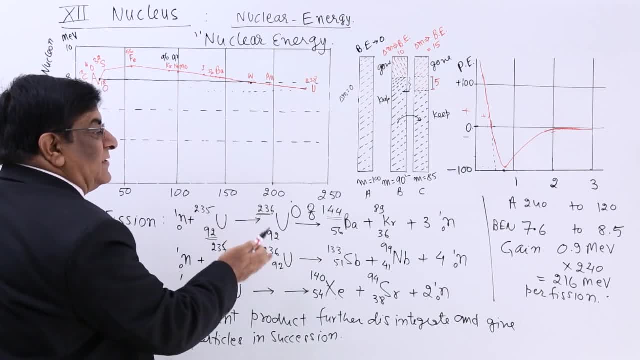 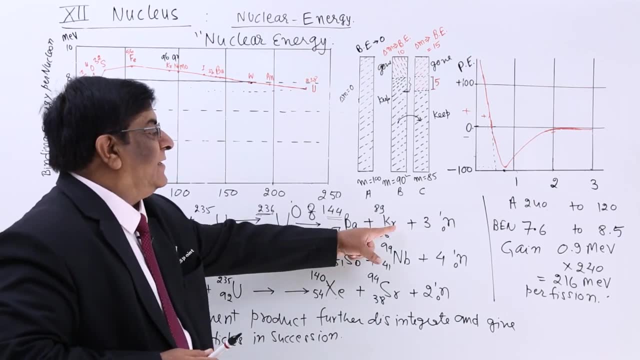 So we write each and every combination that these are the three possibilities. The maximum percentage of uranium breaks into this: barium and krypton. Less than that is this And less than that is this, And a very small portion also breaks into this. 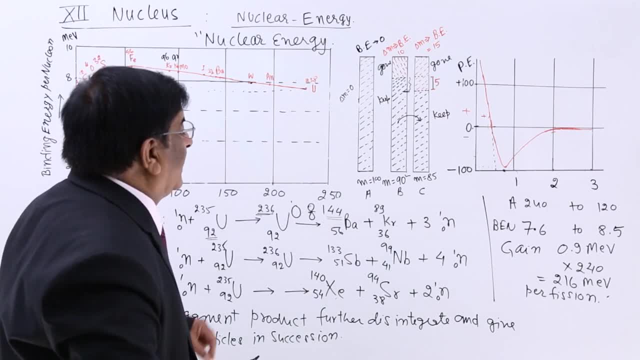 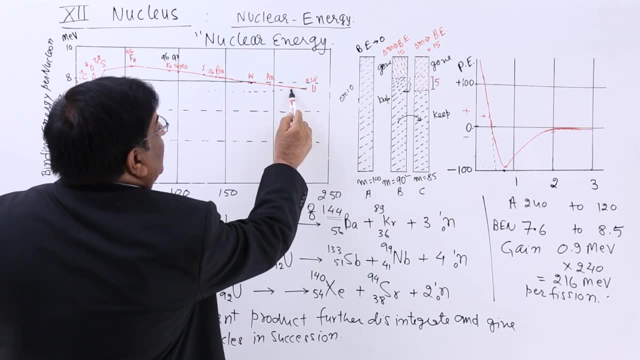 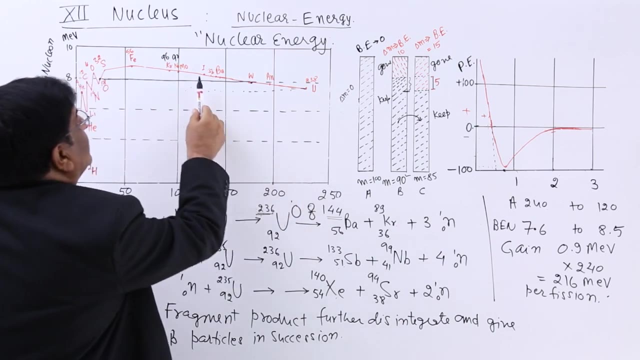 This is what we observe Now, when this breakage takes place, see, Uranium has energy which is 7.6,, almost 7.6.. Now, krypton barium: here is krypton-86.. Here you see. 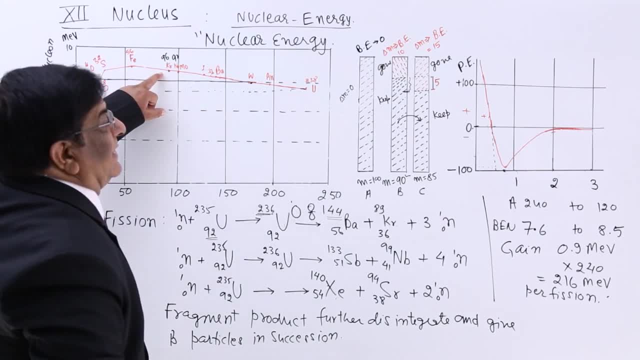 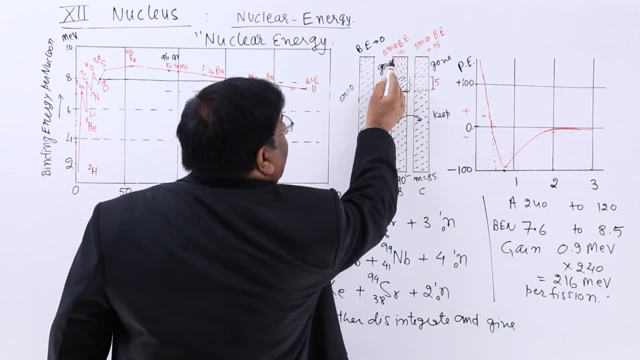 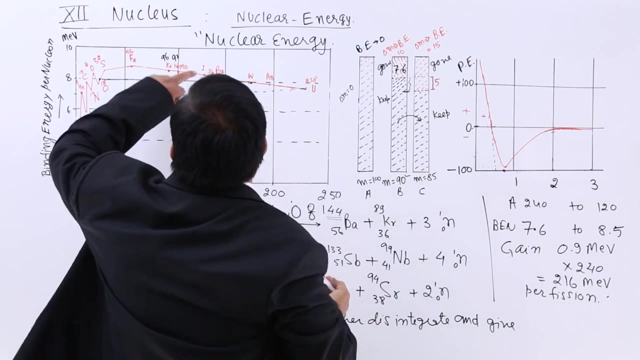 How much energy that is Ben it has. It has Ben-8.5.. This is 7.6.. This is uranium-7.6.. This is say, we take it as krypton and this is 8.5, 8.5.. 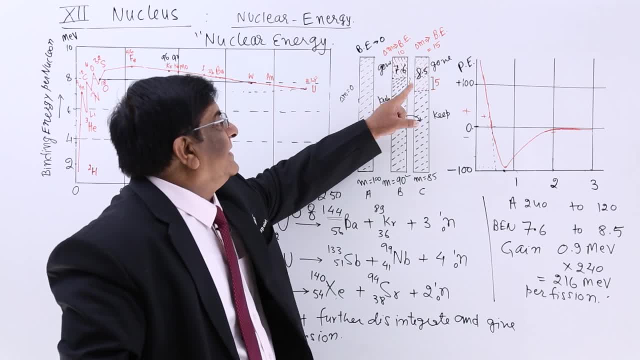 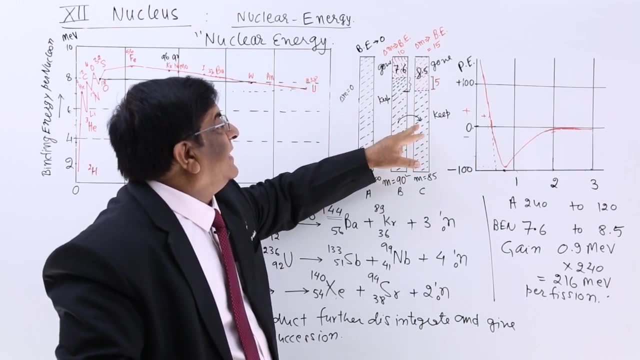 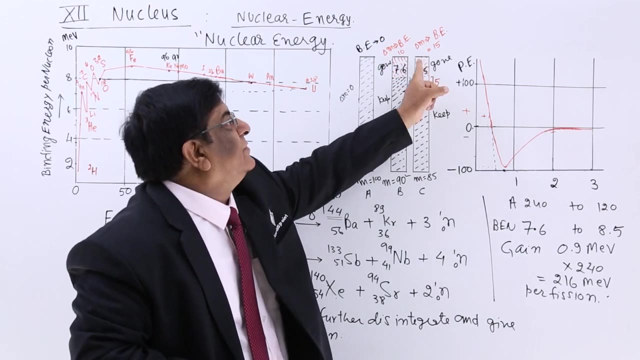 Now, if this nucleoid of 7.6 is converted to this nucleoid of 8.5, we gain so much energy. So much energy is radiated out. This much energy is radiated out, This, out, out out. 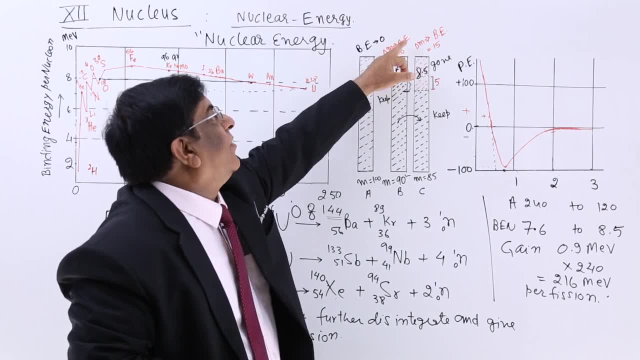 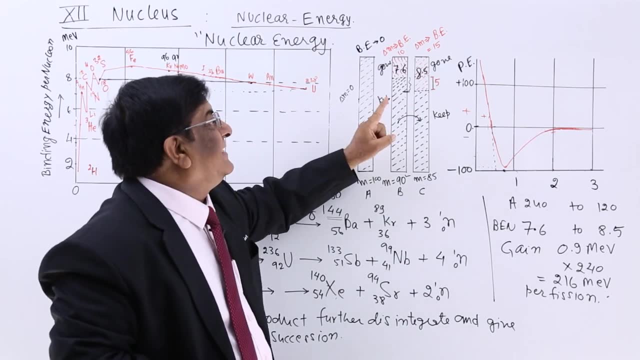 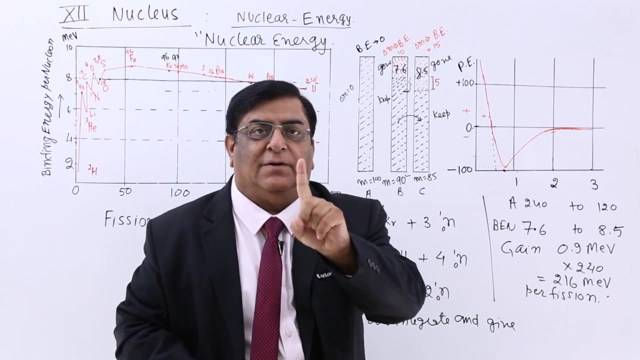 This was already out- 7.6.. Was already binding energy for uranium. Now this energy for krypton become 8.5.. So we get energy, How much We get energy: 0.9.. That is our gain for one, for one nucleoid. And how many nucleoid it has: Nearly 240,, roughly So 240,. how much energy we get: 216 million electron volt for one nucleus of uranium, Because one nucleus has got nearly 235 to 240 nucleoid And every nucleoid the energy level decrease.